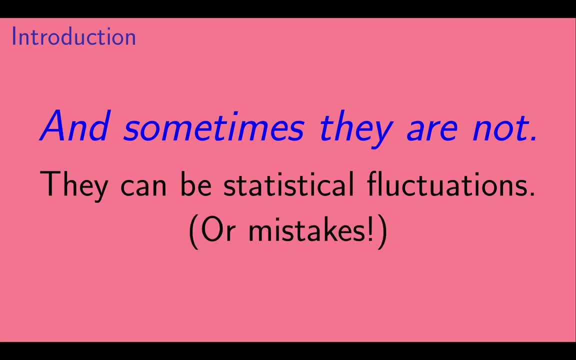 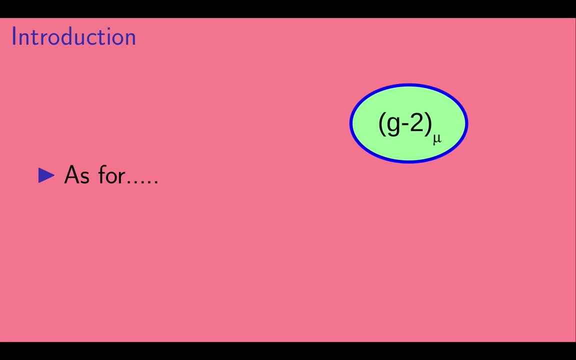 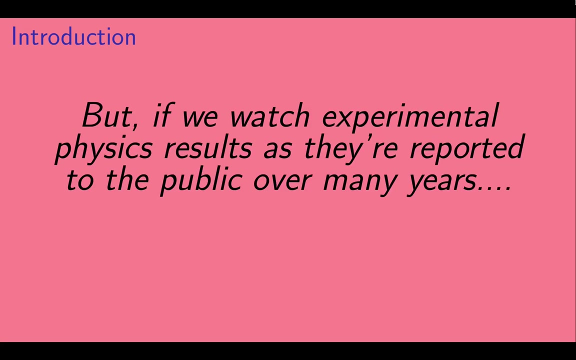 fluctuations or, unfortunately, sometimes even mistakes. As for muon g minus two, the W mass and those flavor anomalies, we will have to wait and see if they are signs of new physics or red herrings. But if we watch experimental physics results as they're reported to the public over many years, we can get a. 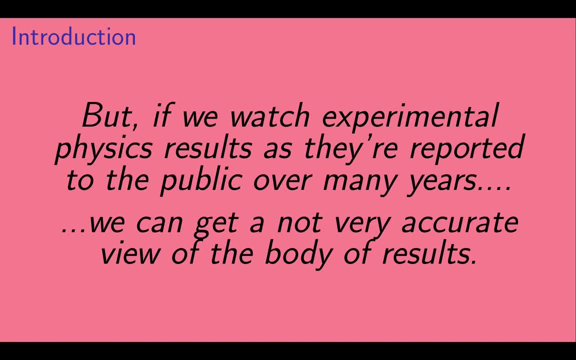 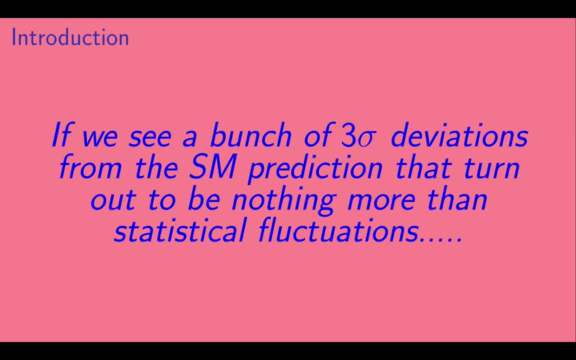 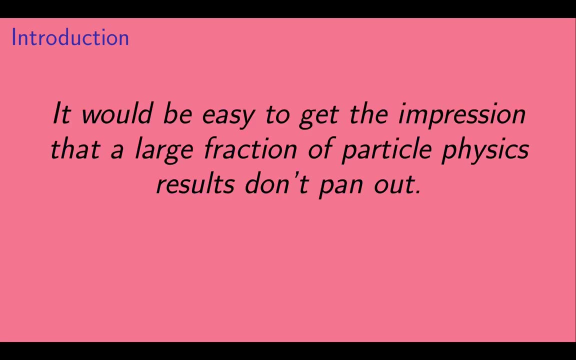 not very accurate view of the body of experimental results. If we see a bunch of three sigma deviations from the Standard Model prediction that turn out to be nothing more than statistical fluctuations, it would be easy to get the impression that a large fraction of particle physics results don't pan out. 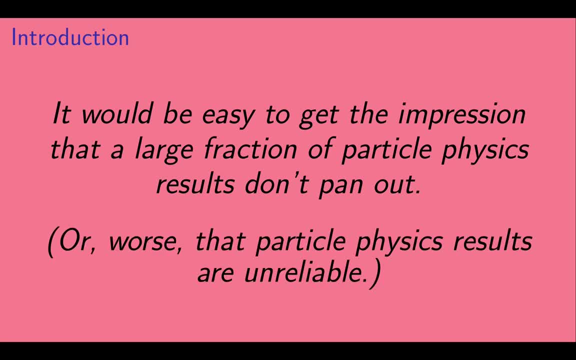 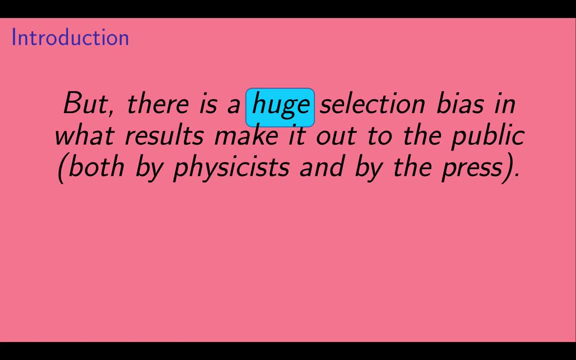 or worse, that particle physics results are unreliable. But this misses an important consideration. There is a huge selection bias in what results make it out to the public and this selection bias is very important because it has to be bias is due to both physicists and the press that report the results Generally. 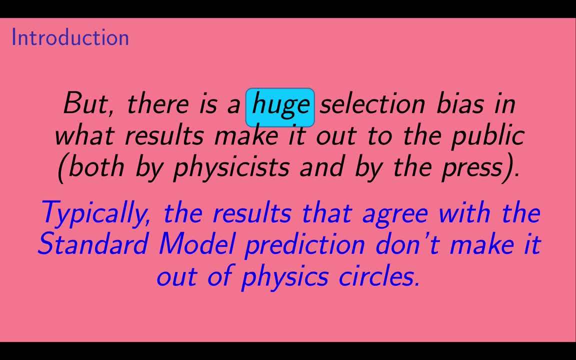 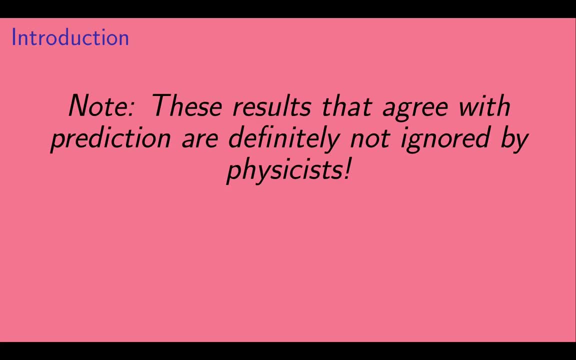 the experimental results that agree with the prediction of the standard model don't make it out of physics circles. Now I should point out that I don't mean that the results that agree with the standard model prediction are ignored by physicists. These results are published, just not publicized widely to non-. 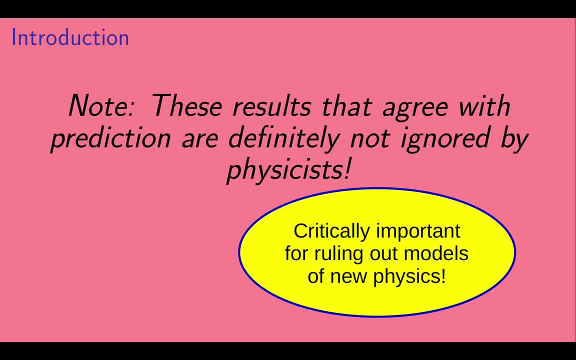 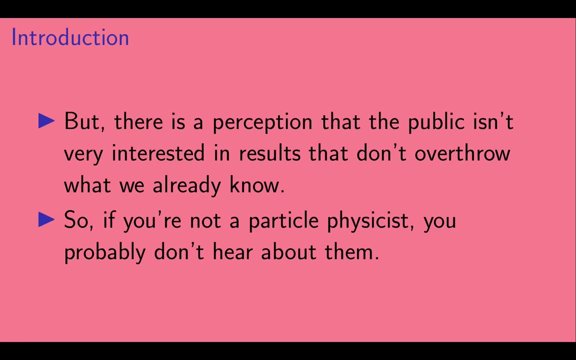 physicists. Those results are critically important to physicists, who use them to rule out models of new physics that have been proposed. But there is a perception that the public isn't interested in results that don't overthrow what we already know. So if you're not a particle physicist, you probably don't hear about. 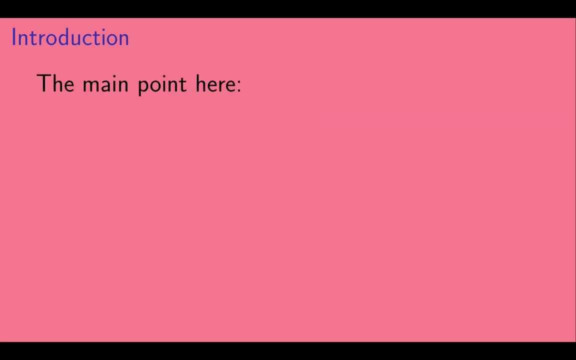 these results. Okay, let me just clarify what the main point is of this video, Even if nothing weird is going on, by which I mean there is no new physics relevant to a particular measurement and the standard model prediction is essentially correct, and if all the 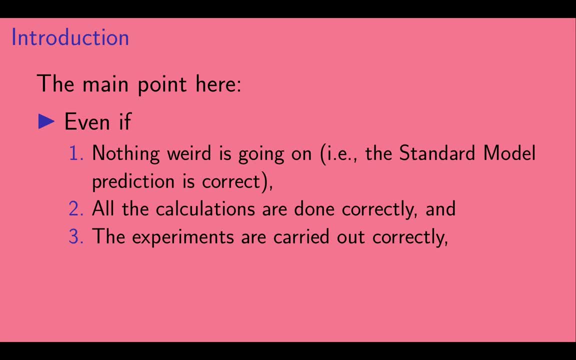 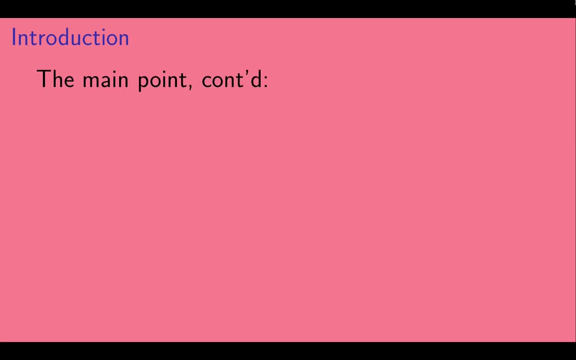 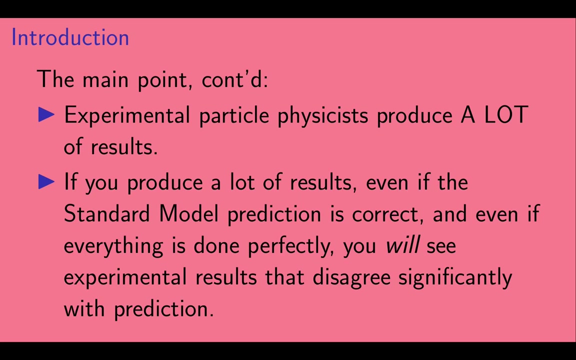 calculations are done correctly and if all the experiments are carried out correctly, some results will disagree significantly with the prediction of the standard model. Additionally, experimental particle physicists produce a lot of results And if you produce a lot of results, even if the standard model prediction is correct, 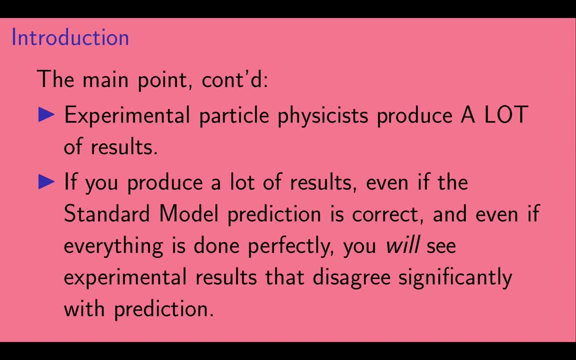 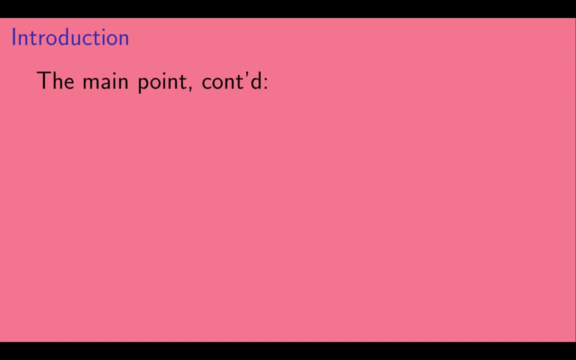 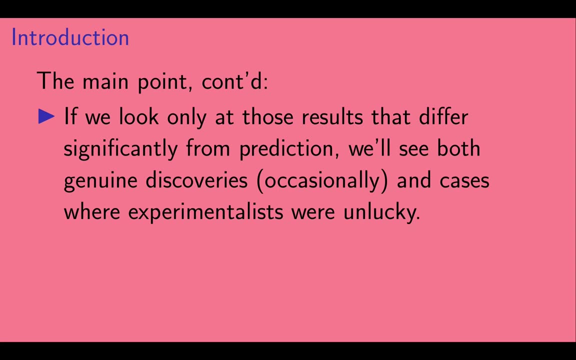 and even if everything is done perfectly, you will see experimental results that disagree significantly with prediction. So if we only see those results that differ significantly from prediction, we'll see both the occasional genuine discovery and cases where experimentalists were unlucky. If, instead, we look at the body of all experimental results, we'll see a very different picture. 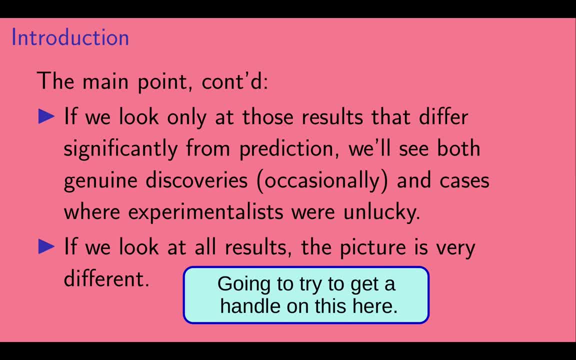 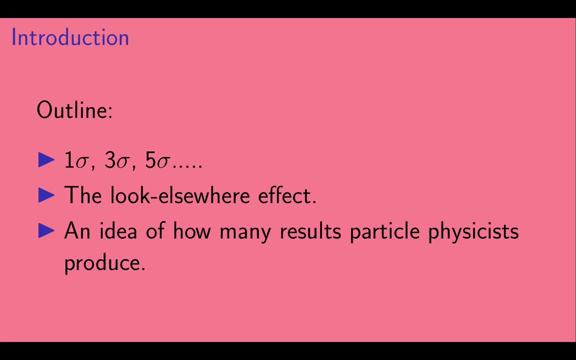 So let's try to get a handle on this here. Okay, So here's a quick example. Okay, so here's an outline of what this video is about. First, we'll talk about sigmas, which is how particle physicists usually quantify the difference. 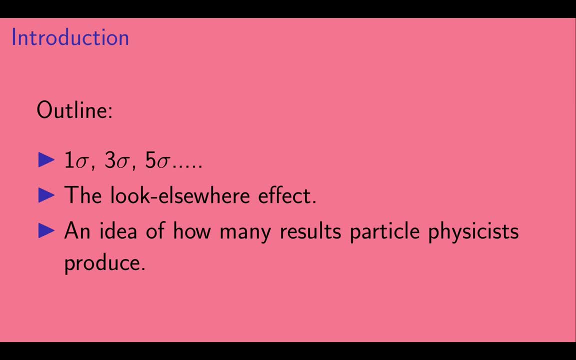 between an experimental result and a theoretical prediction. Then we'll talk about the look elsewhere effect And finally we'll try to get an idea of how many results particle physicists produce in a year. Okay, let's start with 1 sigma, 3 sigma, 5 sigma. 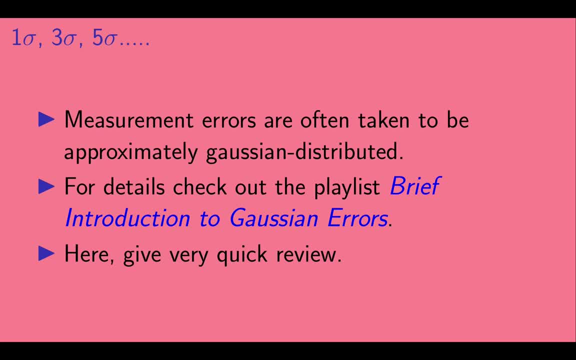 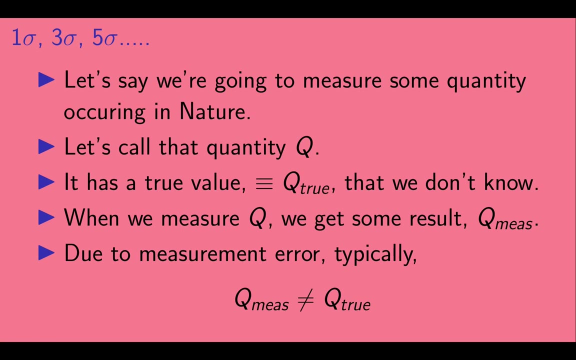 Measurement errors are often taken to be approximately Gaussian distributed. For details check out the playlist. Brief Introduction to Gaussian Errors. Here we will just give a quick review. Let's say we're going to measure some quantity occurring in nature. Let's call that quantity Q. 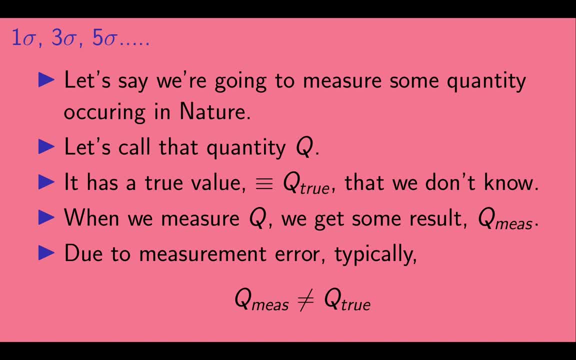 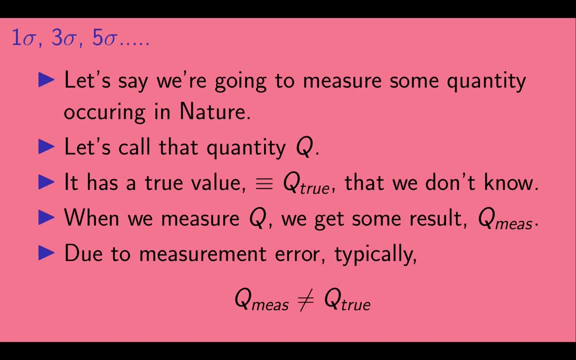 We don't know Q true. When we measure Q, we will get some result of our experiment, which we'll call Q measured. Measurements aren't perfect, though, and there are measurement errors. Thus, typically, Q measured does not equal Q true. Now let's ask: how do we measure Q? 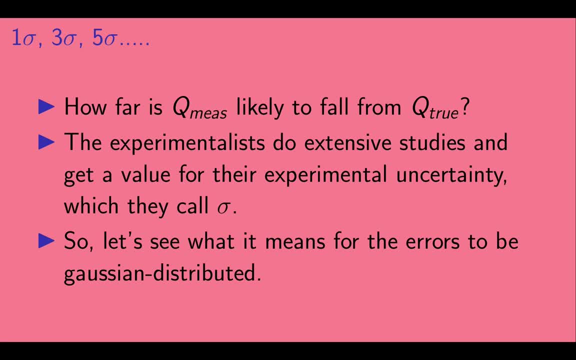 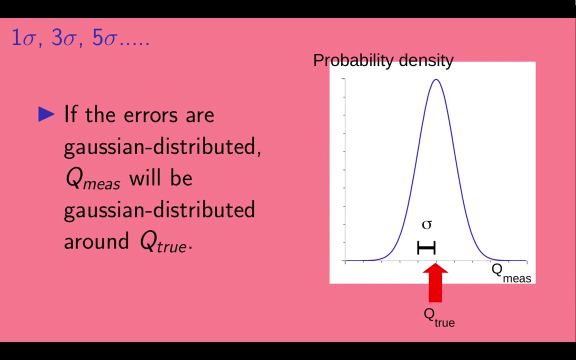 How far is Q measured likely to fall from Q? true, The experimentalists do extensive studies and get a value for the experimental uncertainty which is called sigma. With this let's see what it means for the errors to be Gaussian distributed. If the errors are Gaussian distributed, Q measured will be Gaussian distributed around. 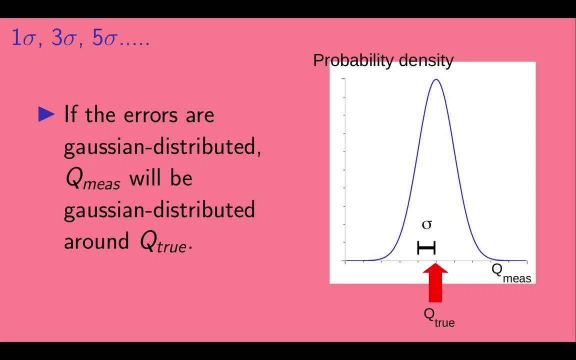 Q true. So on the right we have a plot of the probability density for the result Q measured. The higher the curve, the more likely Q measured is to fall in that area. Q measured is very likely to fall near Q true and very unlikely to fall very far away from. 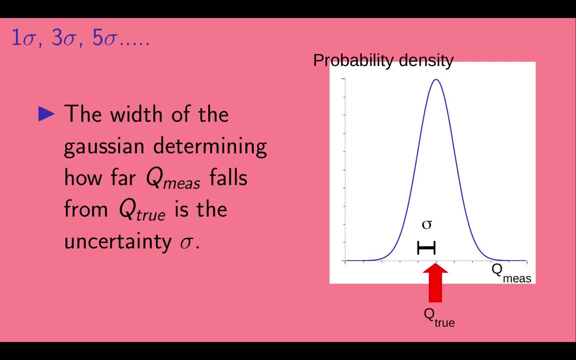 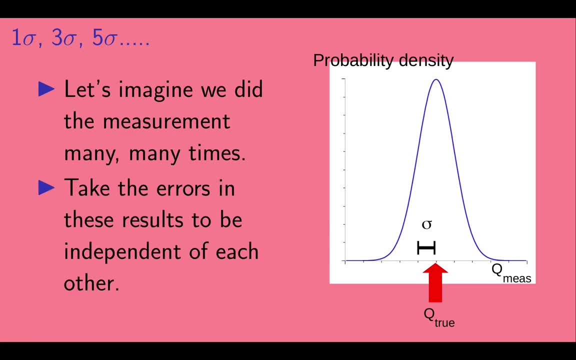 it, The width of the peak. The width of the peak is the uncertainty sigma determined from studies by the experimentalists. Now let's imagine that we did the experiment many, many times. We will take the errors in these results to be independent of each other. 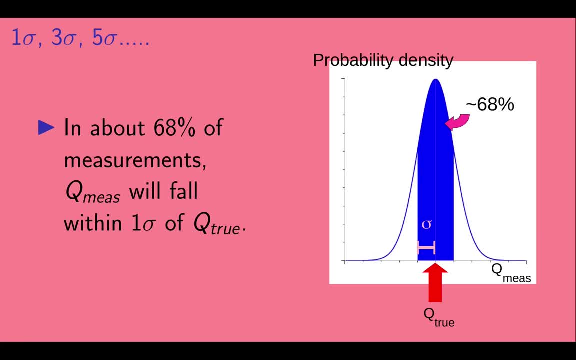 In about 68% of measurements Q measured will fall within one sigma of Q- true. In about 95% of measurements Q measured will fall within two sigma of Q true, And in about 99.7% of cases it will fall within three sigma. 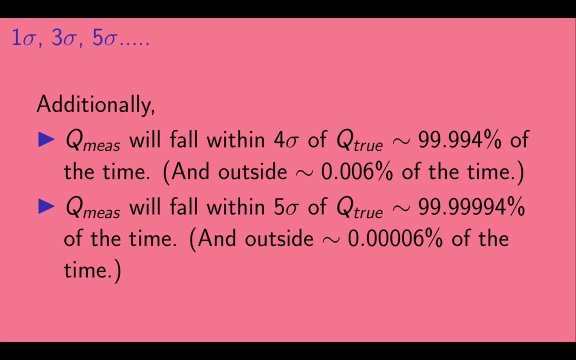 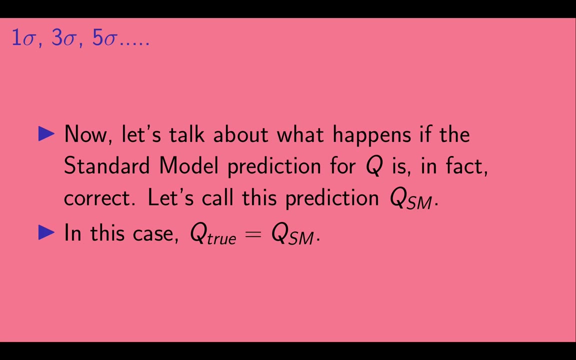 Additionally, it will fall within four sigma- about 99.994% of the time, and within five sigma- about 99.99994% of the time. Okay, Now Let's talk about what happens if the standard model prediction for Q is in fact correct. 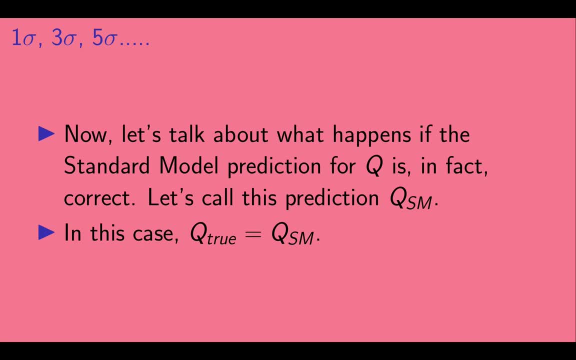 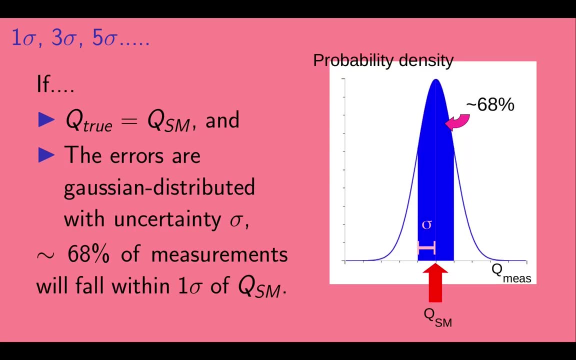 We will call the standard model prediction QSM. So here Q true equals QSM. If Q true is QSM and the errors are Gaussian distributed with uncertainty sigma, then approximately 68% of measurements will fall within one sigma. Okay, We will call the standard model prediction QSM. 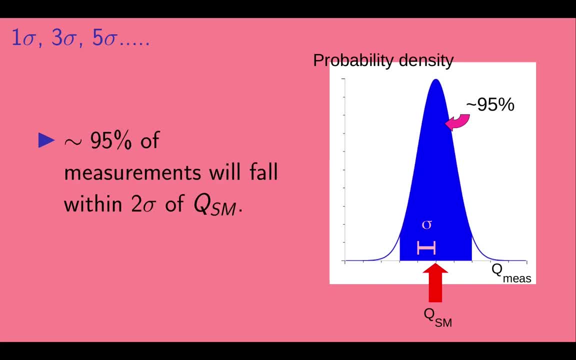 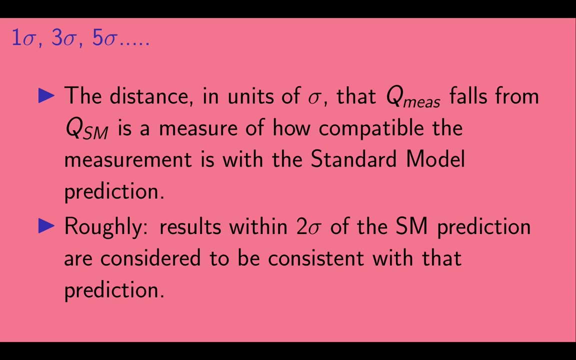 And similarly about 95% will fall within two sigma of QSM and about 99.7% will fall within three sigma of QSM. The distance in units of sigma that Q measured falls from QSM is a measure of how compatible the measurement result is with the standard model prediction. 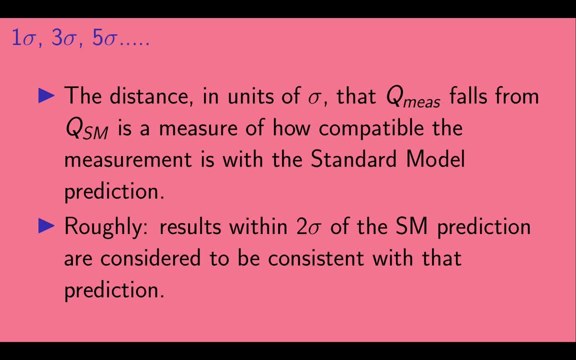 Okay, Let's take a look. Okay, So the standard model prediction is a measure of how compatible the measurement result is with the standard model prediction. Roughly speaking, we tend to say that results within two sigma are consistent with the standard model prediction. 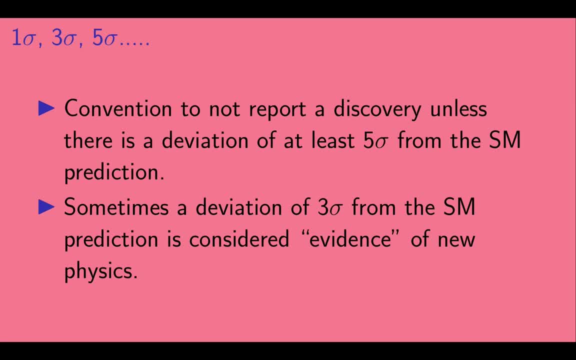 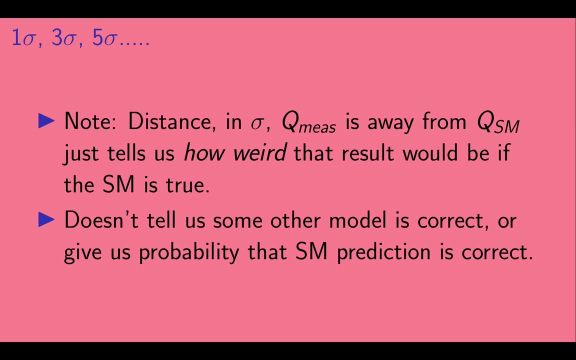 Also, there is a convention in particle physics to not declare discovery unless the deviation is at least five sigma from the standard model prediction, And sometimes a deviation of three sigma is considered evidence of new physics. I should point out that the distance in sigma that Q measured is away from QSM only tells. 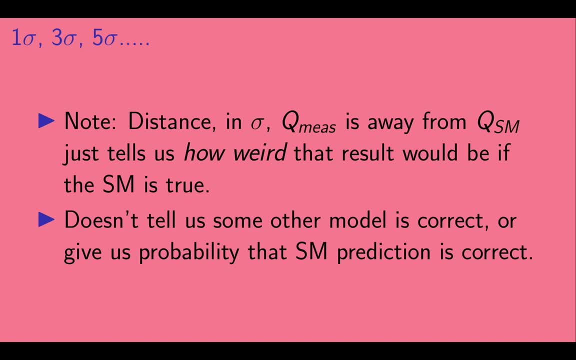 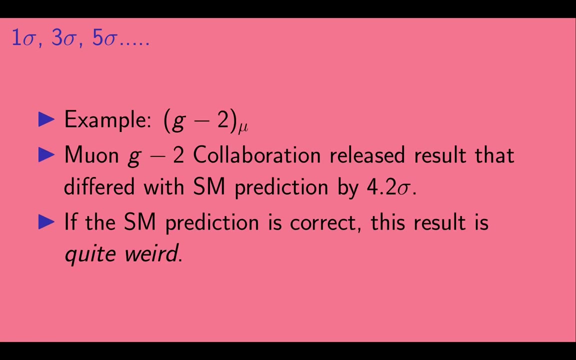 us how weird the result is: if the standard model prediction is true, It doesn't tell us that some other model is correct, or even give a probability that the standard model prediction is correct. Okay, Okay. For example, let's look at the recent measurement of muon: g minus two. 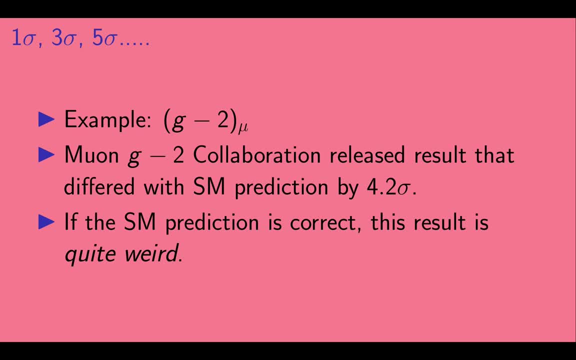 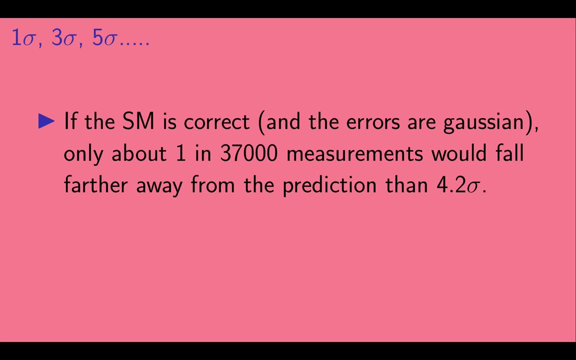 It differs from the standard model prediction by 4.2 sigma. If the SM prediction is in actuality correct, then this result is quite weird. If the standard model is correct and if the errors are in fact Gaussian, only about one in 37,000 measurements would fall. 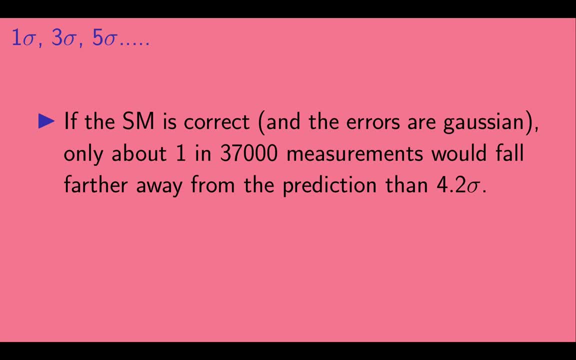 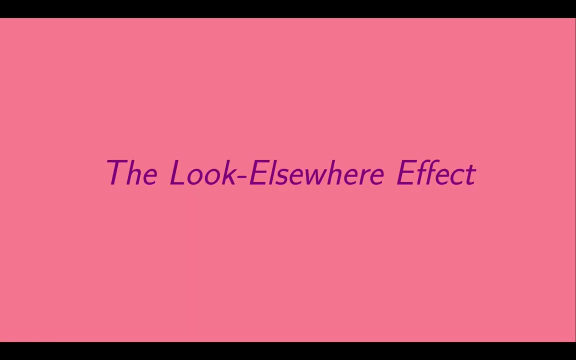 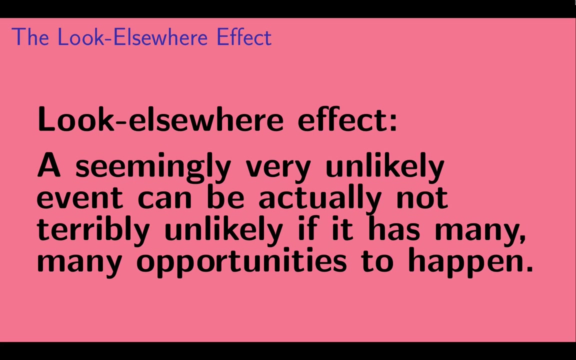 Okay, If the average of muon g minus two is zero, then the number of measurements would fall farther away from the prediction than 4.2 sigma. But, and this is important, one in 37,000 is not zero, And this brings us to the look elsewhere effect. 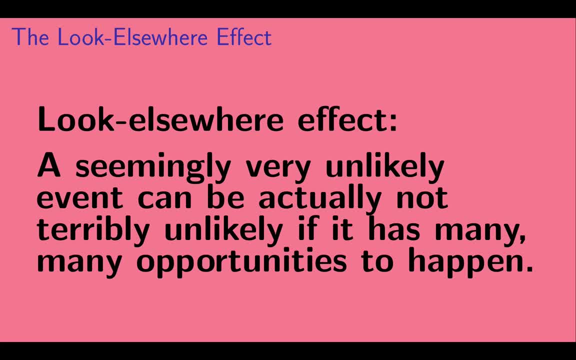 The look elsewhere effect, also known as the multiple comparisons problem, can be stated as follows: A seemingly very unlikely event can be actually not terribly unlikely if it has many, many opportunities to happen. Assuming Gaussian errors, Q measured will fall more than 3 sigma. 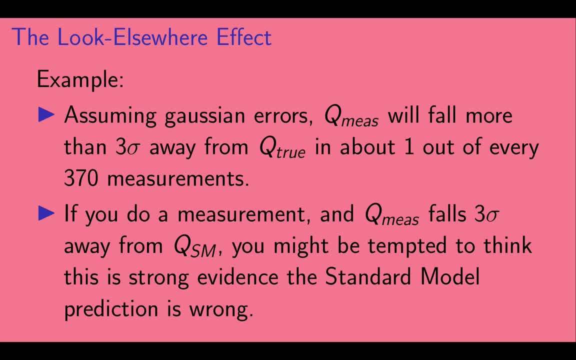 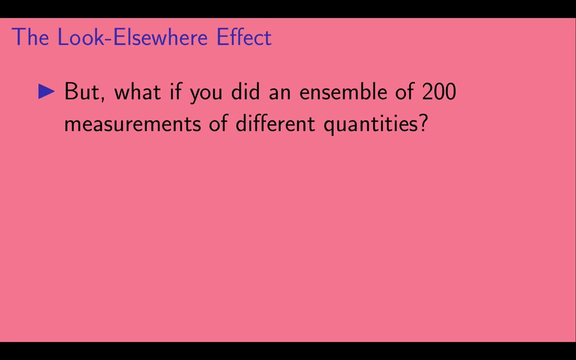 away from Q. true, in about one out of every 370 measurements. If you do a measurement and Q measured falls 3 sigma away from QSM, you might think this is strong evidence that the standard model prediction is wrong. But what if you did an ensemble of measurements? Let's say you measured 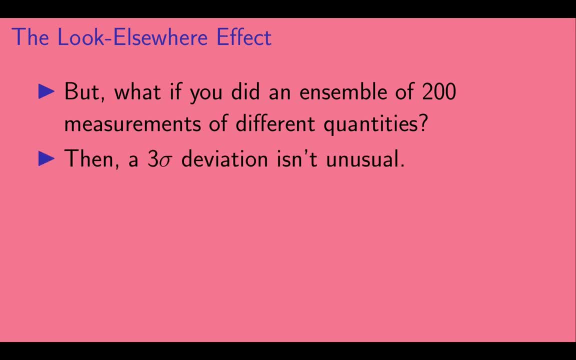 200 different quantities, Then a 3 sigma deviation from prediction isn't unusual. In fact, it's downright normal. This will happen 31% of the time. In fact, it's downright normal. In fact, it's downright normal. This will happen 31% of the time. 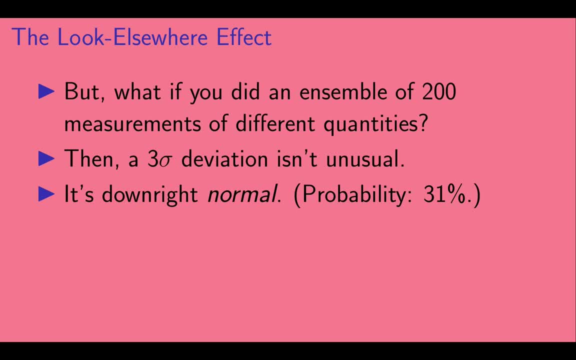 In fact you could have more than one 3 sigma deviation. The probability of having two 3 sigma deviations is not that small- about 8.5%- And the probability of having three of them is 1.5%. That's small, but it's not tiny, So a 3 sigma deviation isn't weird at all. 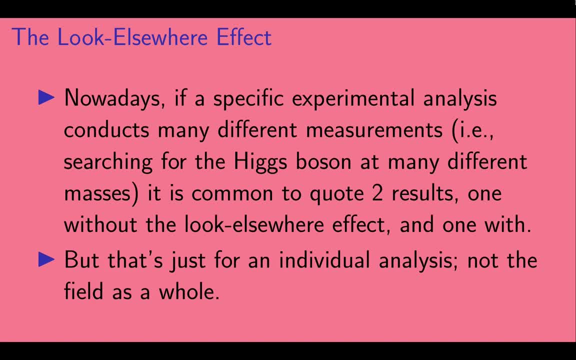 These days, if a specific experimental analysis conducts many different measurements, for example searching for the Higgs boson at many different masses, it is common to quote two results, one without taking the look elsewhere effect into account and one with it. But that's just for an individual analysis, not the field as a whole. 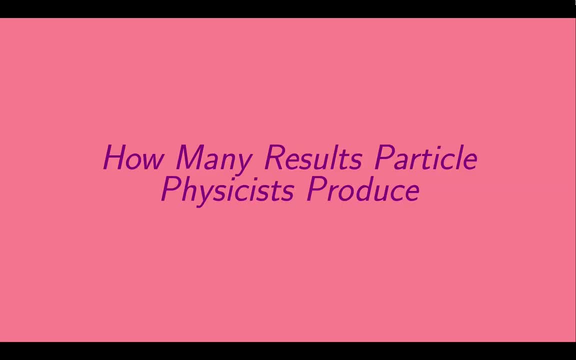 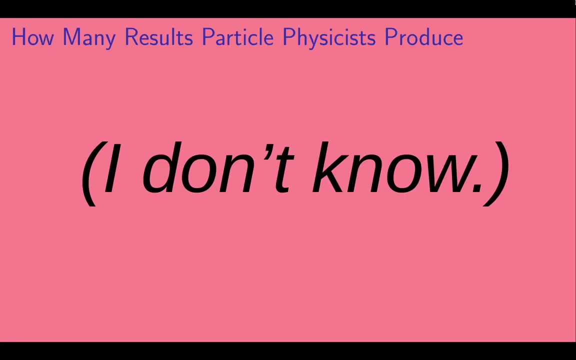 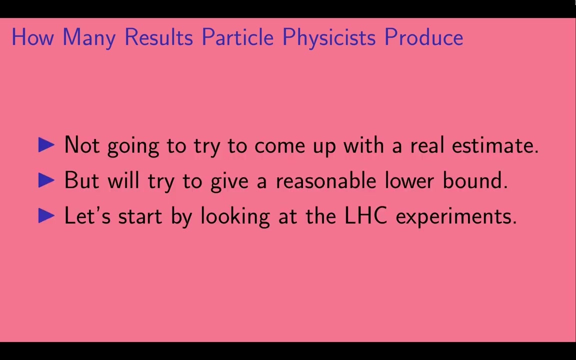 So now it's time to ask how many results particle physicists produce, say, in a year. I don't know the answer to this, But it's a lot. I'm not going to try to come up with a real estimate. Instead I'll try to give a reasonable. 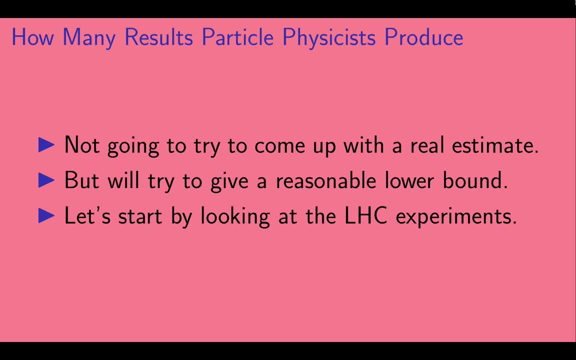 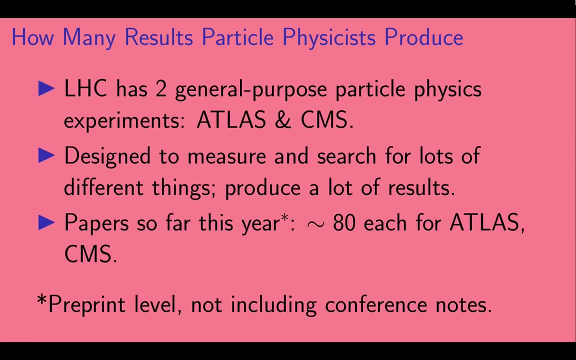 lower bound on the number of experimental results in a year. Let's start by looking at the LHC experiment. Let's start by looking at the LHC experiment. LHC has two general-purpose particle physics experiments: ATLAS and CMS. These experiments were designed to measure and search for lots of different things. 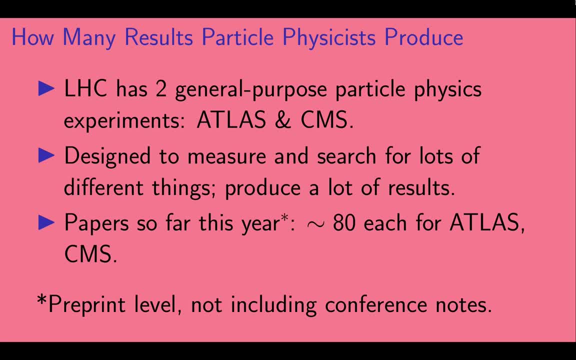 and, as a result, they produce a lot of physics results. So far this year, ATLAS and CMS have both produced around 80 papers each. That might sound like 80 experiments, but it's not. It's a lot of experimental results. 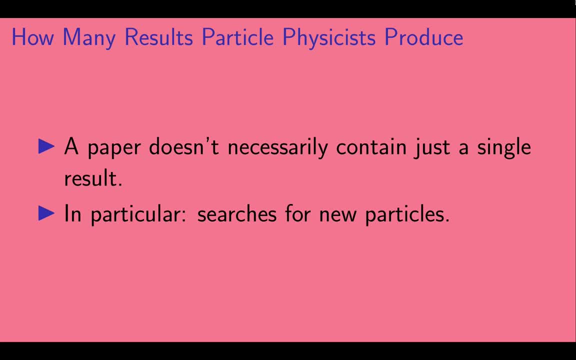 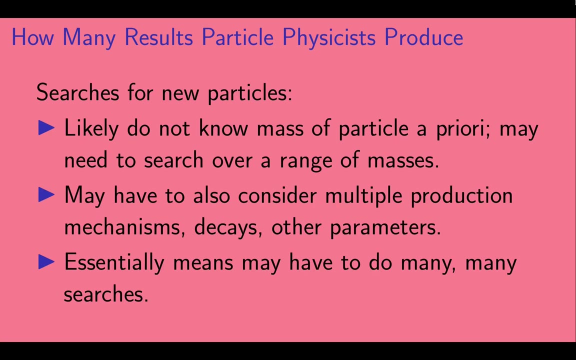 But a paper doesn't necessarily contain just a single result. To illustrate this, let's think for a moment about searches for new particles. When looking for a new particle, we likely do not know the mass of that particle a priori, So we might need to search over a range of masses. 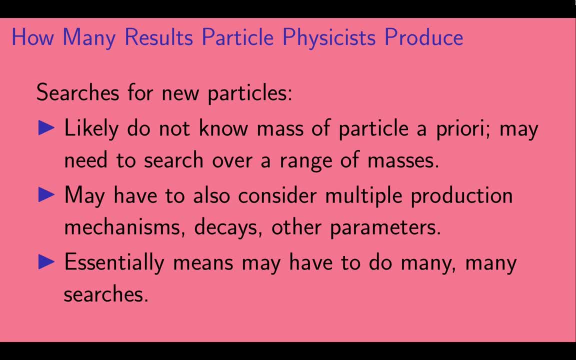 Looking for a particle that has a mass of one particle. we might need to search for a range of masses. Looking for a particle that has a mass of one particle, we might need to search over a range of masses, Looking for a particle that has a mass of 1 TeV. 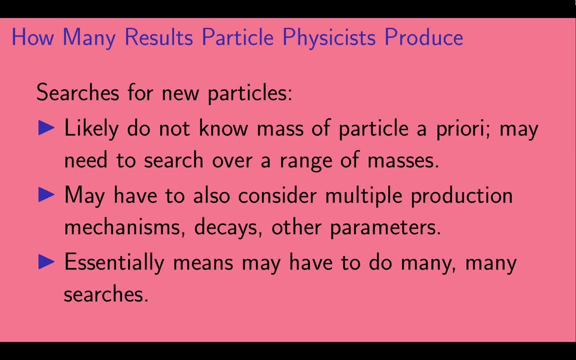 And looking for the same particle but with a mass of 2 TeV can mean producing essentially separate measurements. Additionally, you have to consider multiple production mechanisms or decays of the particle or other theoretical parameters. This means that you might have to effectively do many, many searches. 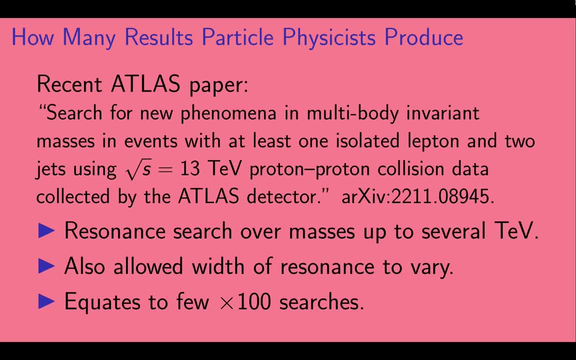 As an example, let's look at this recent experiment. look at this recent paper from Atlas. This paper describes a search for a new particle with a mass anywhere in a range over several TeV. Additionally, the decay width of the particle was allowed to vary. This paper equates to doing a few. 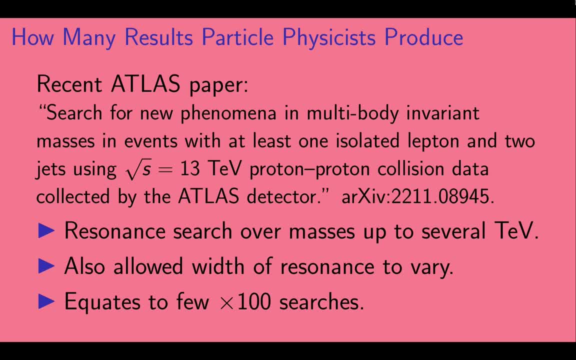 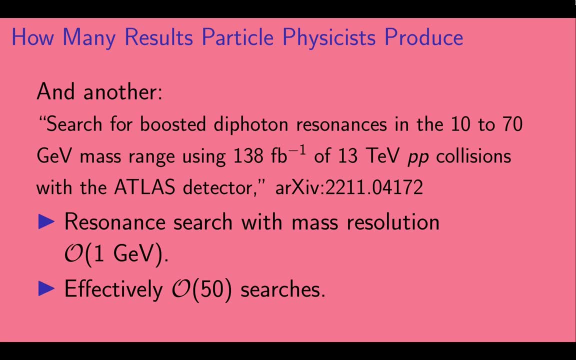 hundred separate measurements. Or we can look at this paper, also very recently put out by Atlas. Here they looked for a new particle whose mass they took to be between 10 and 70 GeV. Their mass resolution was of order 1 GeV, so this: 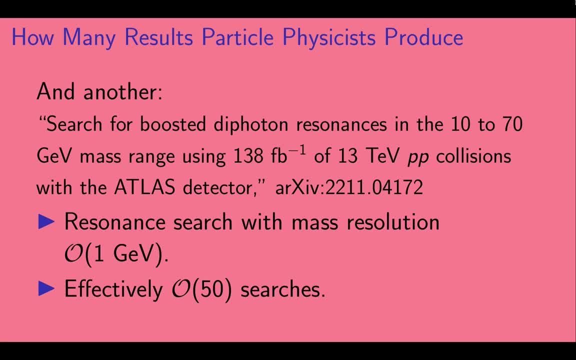 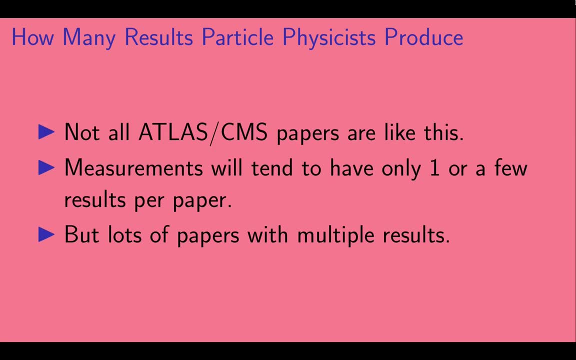 paper effectively contained of order 50 separate measurements. Now, not all Atlas and CMS papers are like this. Papers whose focus is on measuring parameters instead of looking for new particles will tend to have only one or a few results per paper. but there are loads of papers. 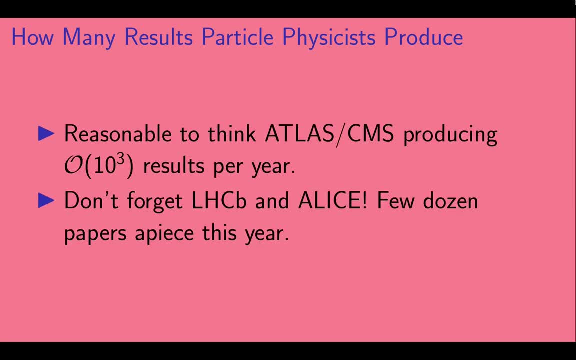 with multiple results. So it's reasonable to think that Atlas and CMS are producing at least of order 1,000 measurements per year. And also, don't forget the other two major experiments at LHC, LHCb and ALIS. They each have. 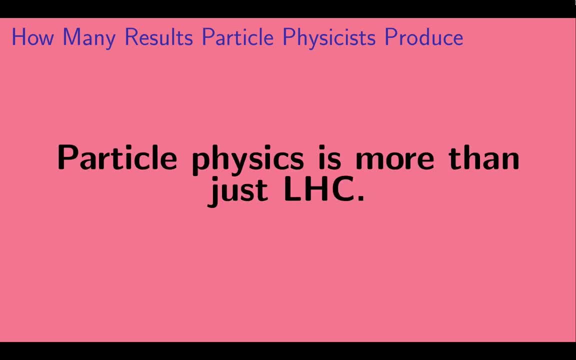 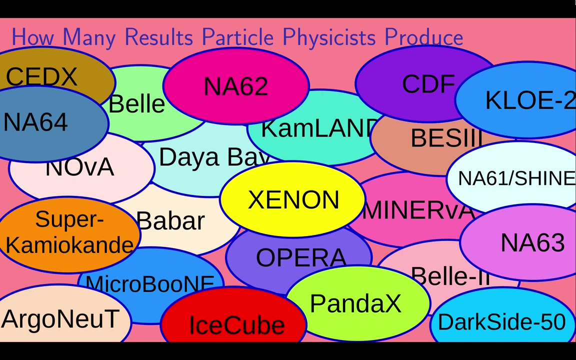 produced a few dozen papers this year. And let's not forget, particle physics is more than just LHC. Here is a goofy cartoon listing a bunch of particle physics experiments. Each of these experiments produced at least one physics paper this year, and some did dozens, And this is definitely not an exhaustive list. So there are lots of. 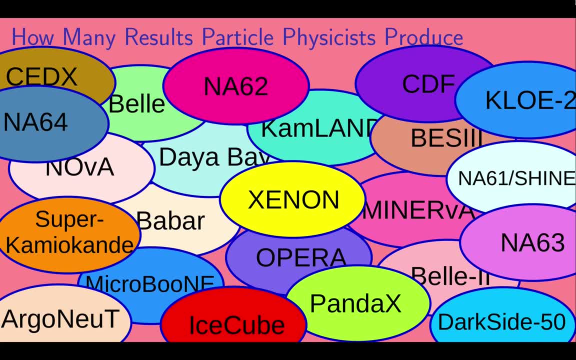 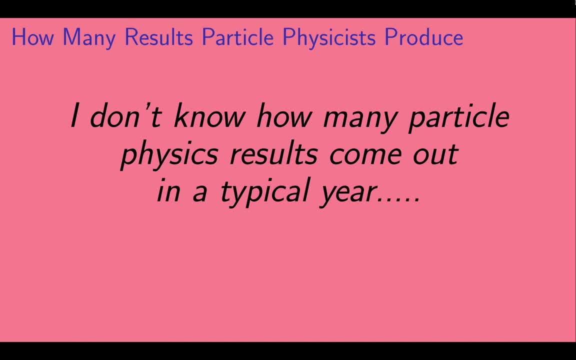 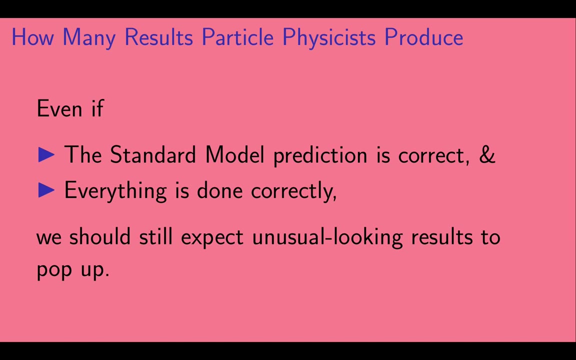 experiments, actively producing these experiments results. So basically, I don't know how many particle physics results come out in a typical year, but I think it's safe to say it's in the thousands. Now, as we pointed out earlier, even if the standard model prediction is correct and even if 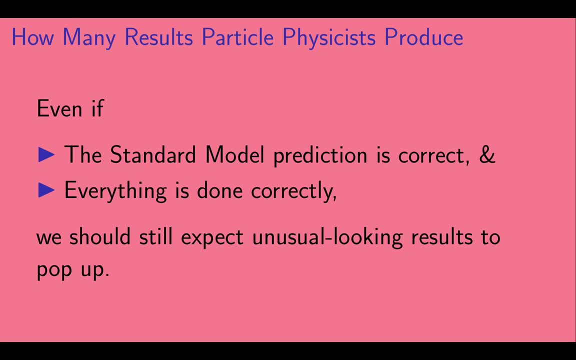 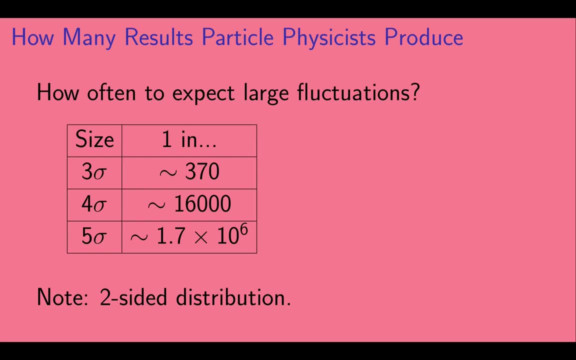 everything is done correctly, we should still expect unusual looking results to pop up. How often should we expect these fluctuations? We should expect to see a three-sigma fluctuation in about one out of every 370 measurements, a four-sigma fluctuation in about one out of every 16,000, and a five sigma fluctuation in.